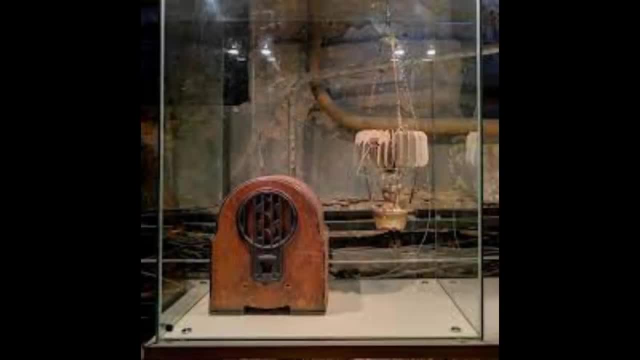 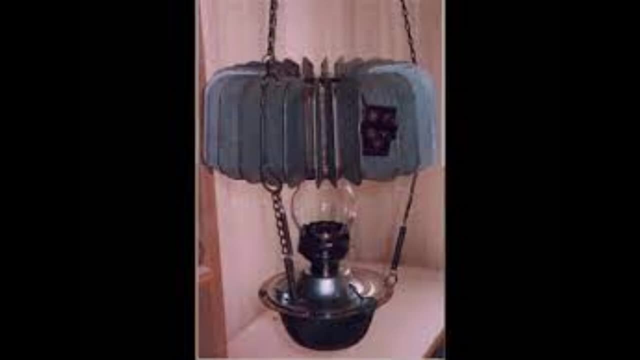 the partisan battery was essentially a Russian invention. it's also called the radio lamp then. it was a mixture of two materials. the inventor used a zinc antimony alloy on one side and constant tan alloy on the other side, which is a nickel alloy. applied the heat from a lamp and it was enough to run a radio. 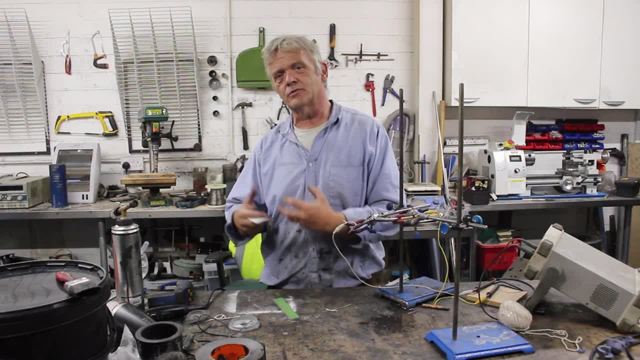 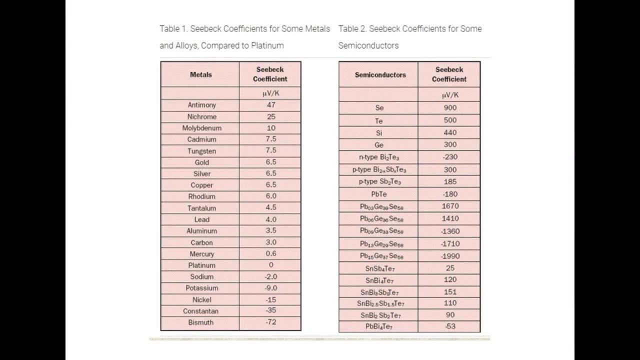 and, and that was a state of play with these thermal junctions, until these things. now you can look up those figures and they're called CBET coefficients. you basically take one from the other and you'll find you have the actual voltage supply per degree centigrade. now they aren't very big, these are in. 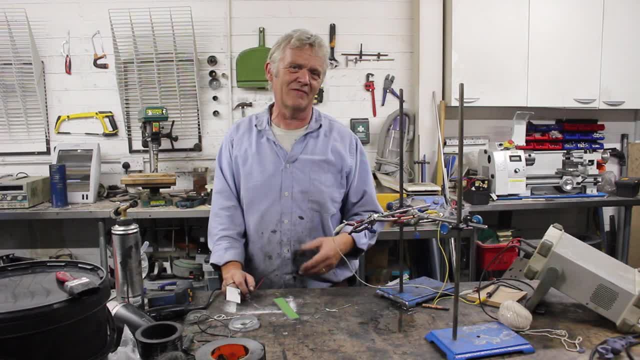 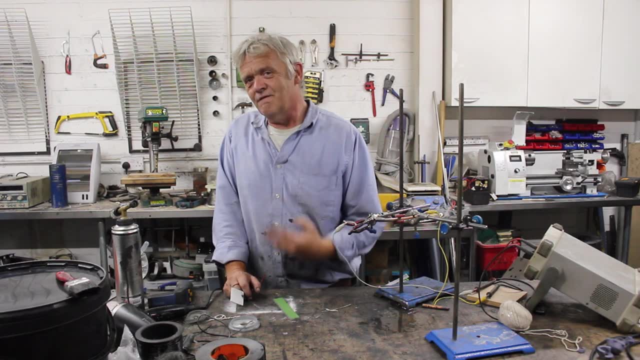 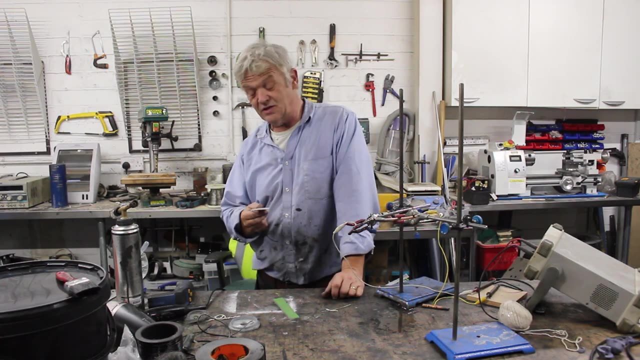 nano volts, which is a thousandth of a micro volt, thousandth of a millivolt, thousandth of a volt. so they're really teeny tiny amounts that you're looking at, but, of course, very, very interesting. now this stuff did really well. small square like that will produce quite a lot for what it actually is, because it's. 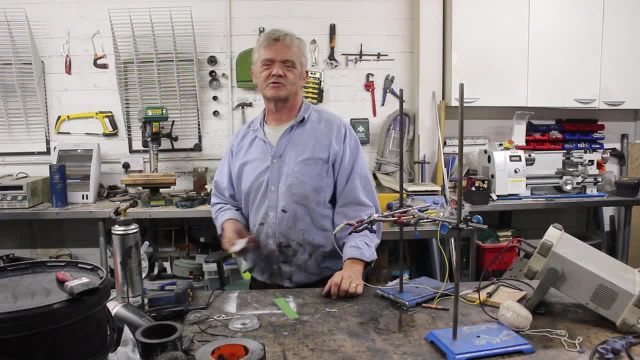 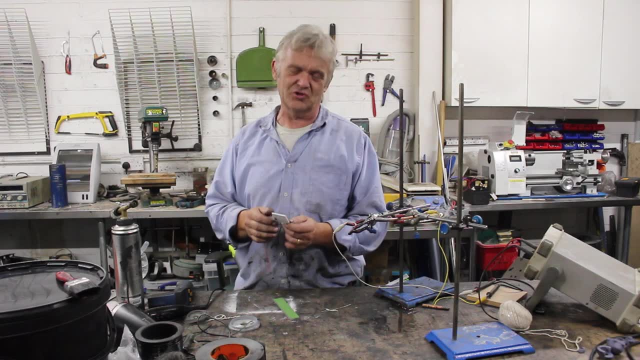 silicon based. it does, however, have its problems. equally, because it's silicon based, it has severe temperature limitations. you can't actually take this above about 200, 300 degrees, so you'll just burn the whole thing out. and so there's a constant search for thermoelectric. 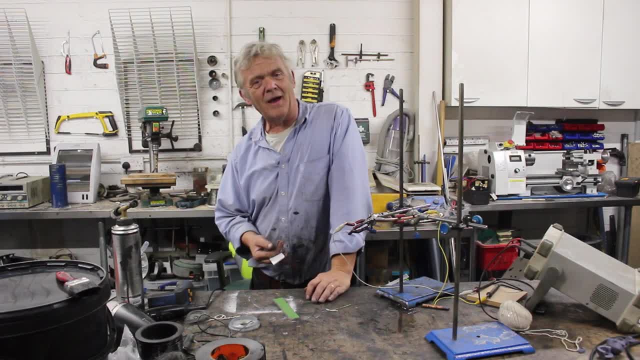 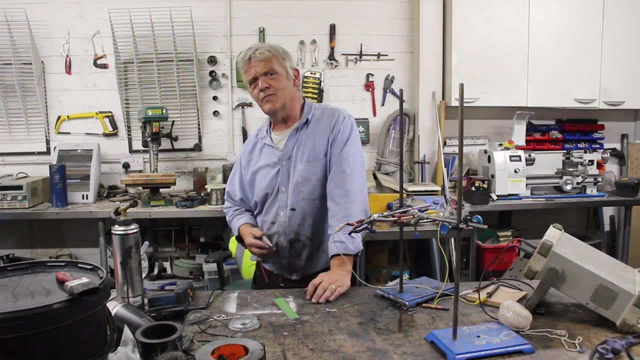 junctions that can develop high powers for relatively relatively low heats, and the common sort of belief in this was the heavier metals, things like bismuth, would do really well. but that was the state of play until a couple of groups, one at Duke University and the other in Montana- 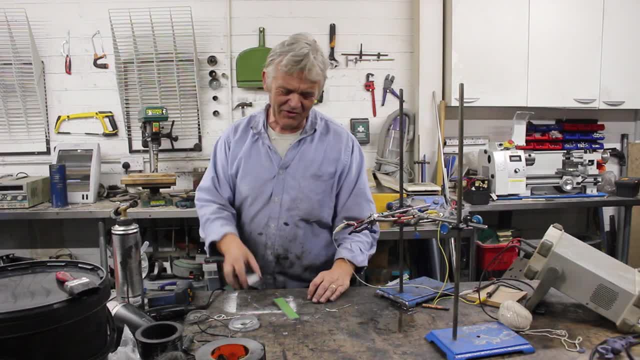 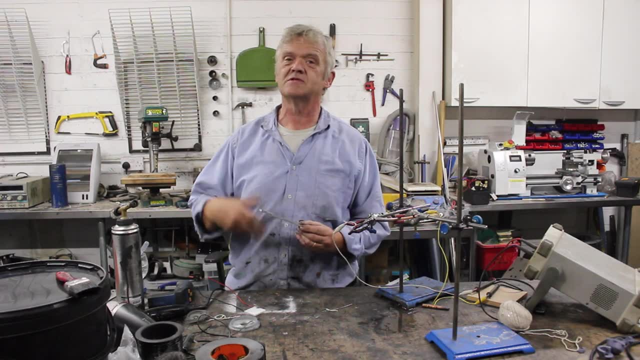 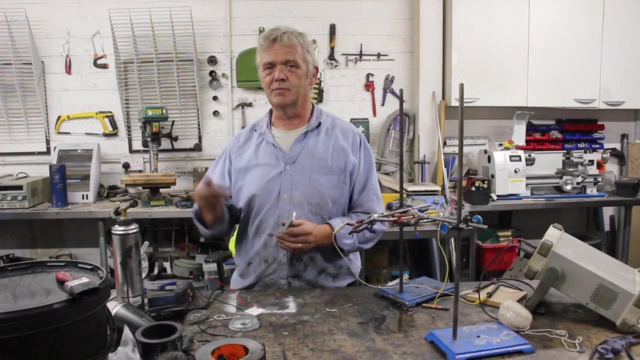 State University disagreed with them. well, they thought was hang on a second. how will this do? yeah, this is a strip of magnesium. actually it's printers plate, so it's a magnesium aluminium alloy. it's about 95 percent magnesium, somewhere between five and seven percent aluminium, and a few of the bits and pieces chopped. 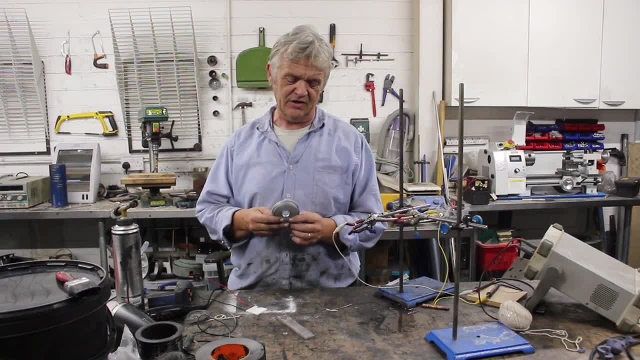 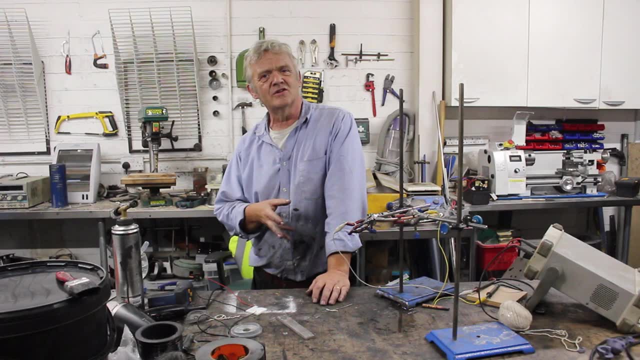 in. this is a bit of pure aluminium, a pure magnesium strip. what the researchers found was that magnesium, magnesium alloys- so magnesium, antimicrobial or magnesium and timonate- worked three to four times better and that was astonishing for everybody because it went against the grain of what everybody. 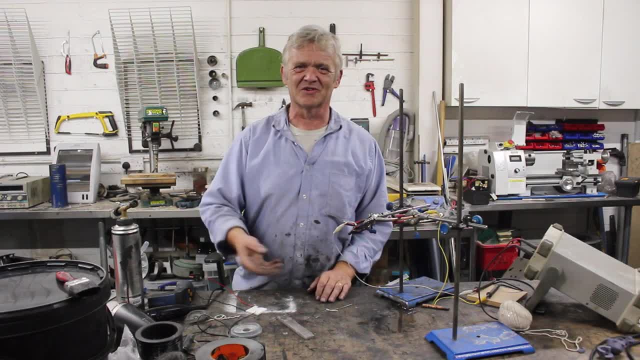 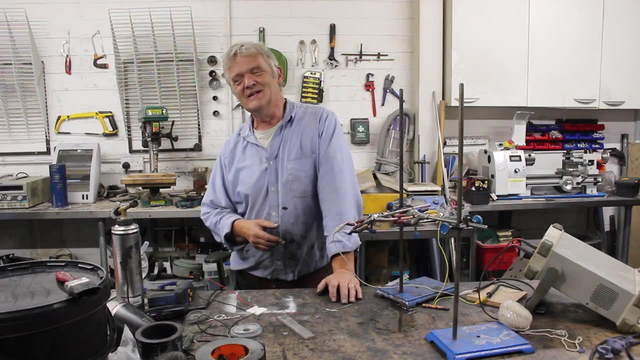 thought, and of course I love that kind of stuff because if you go against the grain, whatever he thinks, and you turn out to be right, I just think that's such a win for all those brave souls who have enough well hoods pad to say no, no, no. 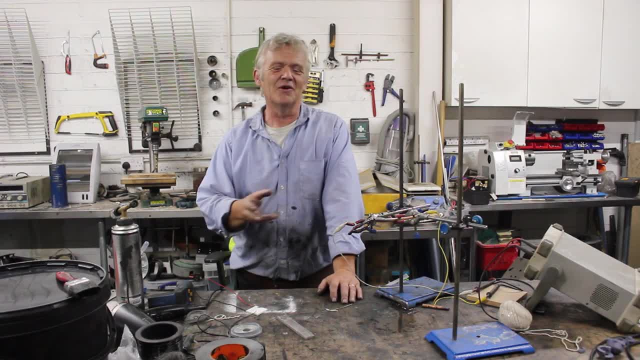 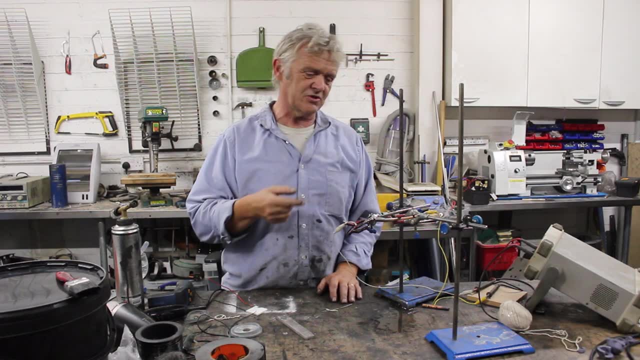 that can't be right. let's try this instead, or maybe even- I don't know- let's give it a go and see. that's spirit- and I find he's got a lot of experience with this, but I find is what usually wins. now, what I've got here is a quick and simple 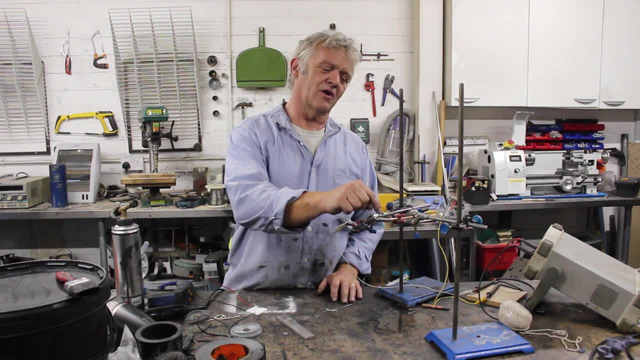 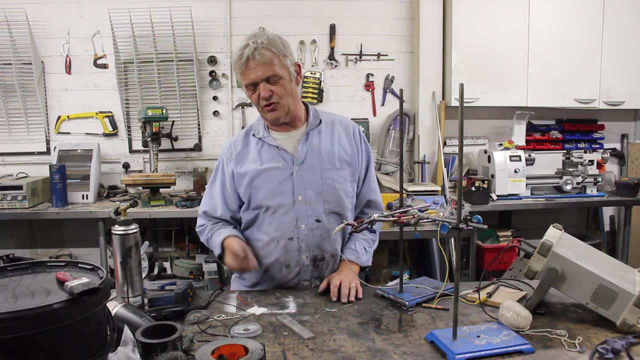 test. we've got a strip of the magnesium ribbon right there making a point contact with this bit of copper. now the sea-back efficient coefficient for copper 6.. I don't know what it is for magnesium, because magnesium of course has a slight drawback if you take it up to temperature when it's a bit of ribbon. 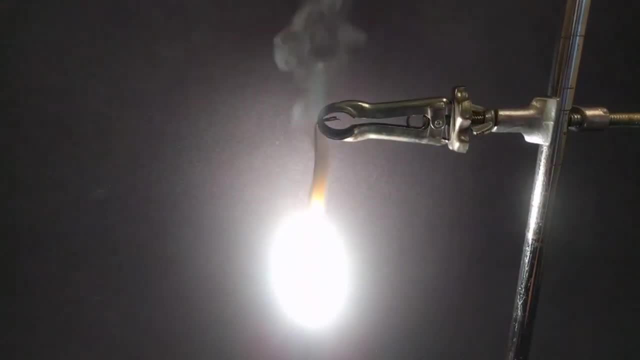 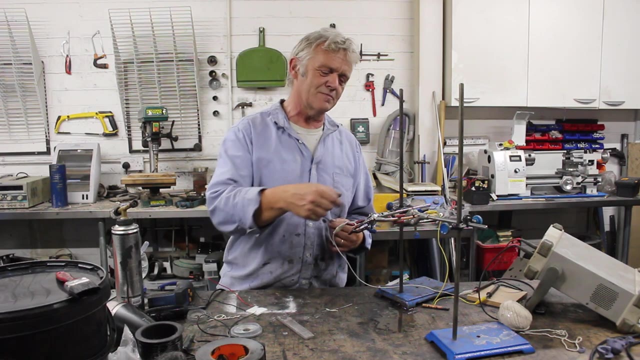 like this. I'm sure we've all seen that science experiment where it burns brilliant white. so you do have to be a bit careful with it and to watch out. it doesn't actually catch fire. so away from the edge a little bit. got a point contact and I'm going to apply. 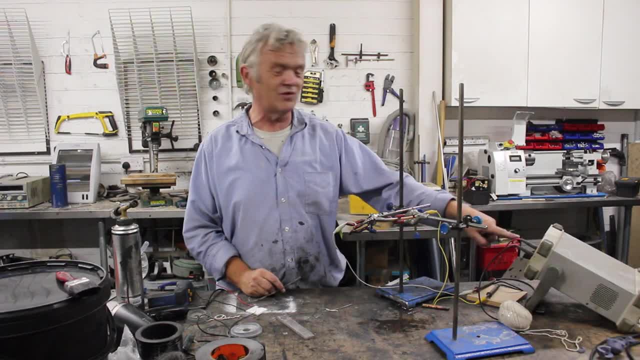 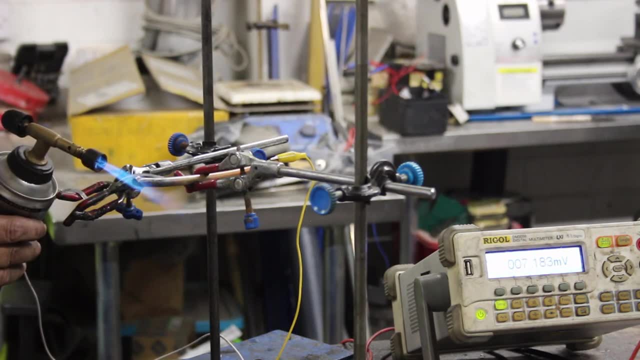 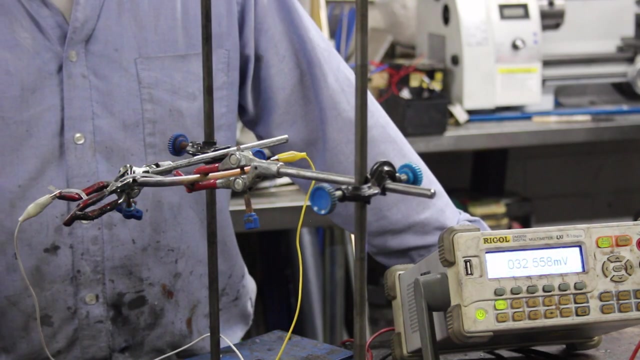 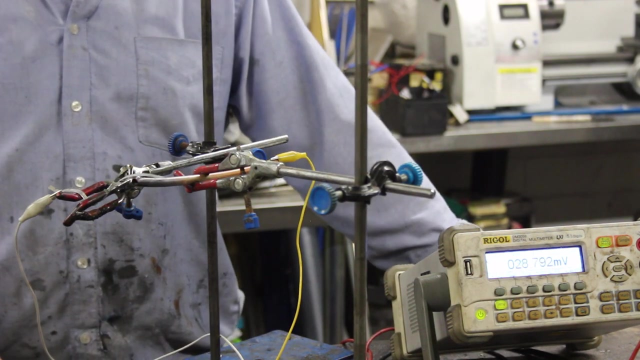 some heat to that copper and we'll see what it does to the voltage which I'm registering here. Now I do have to be a little careful with it because I don't want to burn that out, obviously, but it registered 150 millivolts, which is phenomenal. Now it's. 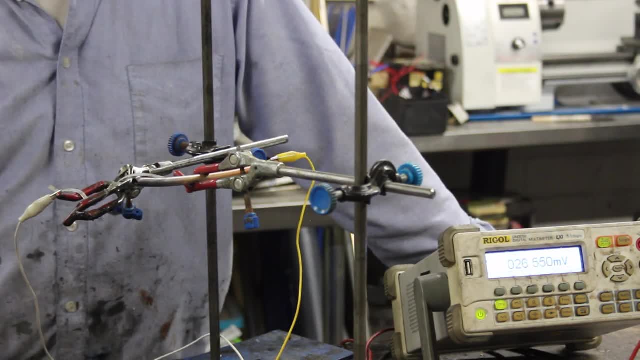 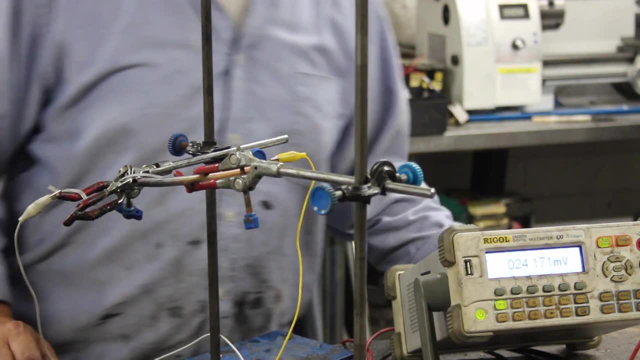 a point contact, so it's not going to produce in huge amounts, but we should be able to produce something out of that. and one way to tell whether we're doing something like that is to put a capacitor in series with it and measure the voltage in parallel with it and measure the voltage across the. 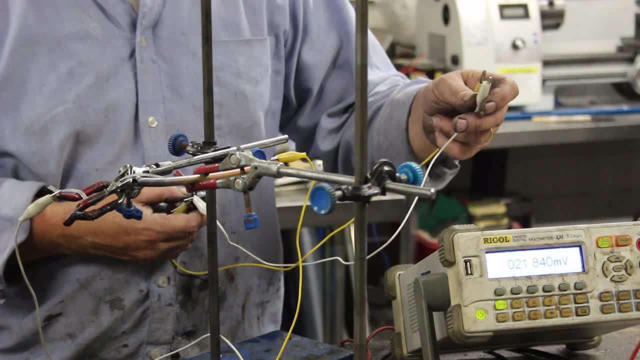 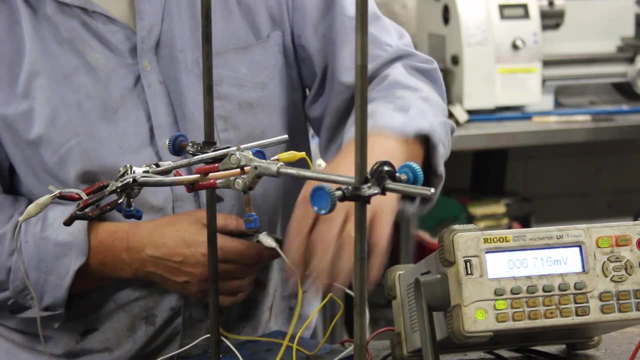 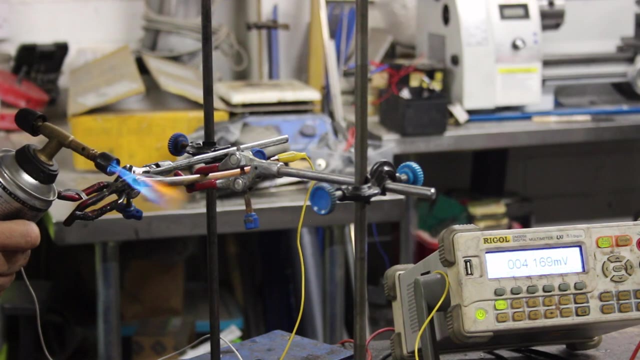 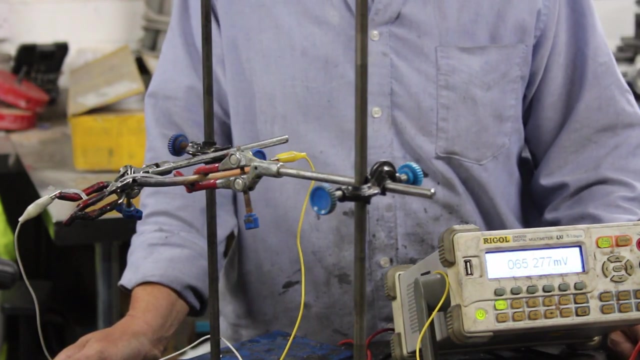 capacitor. Because if we can do that, then we are actually putting energy into the capacitor and we're measuring that energy being generated. So let's put a capacitor across those two lines and do that again. plus We've got about 50 to 60 millivolts- 64 milivolts- across that capacitor from. 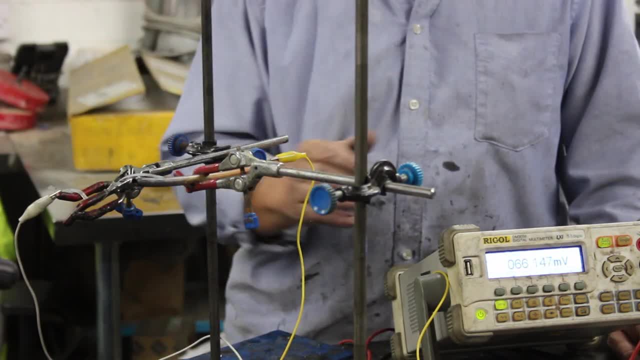 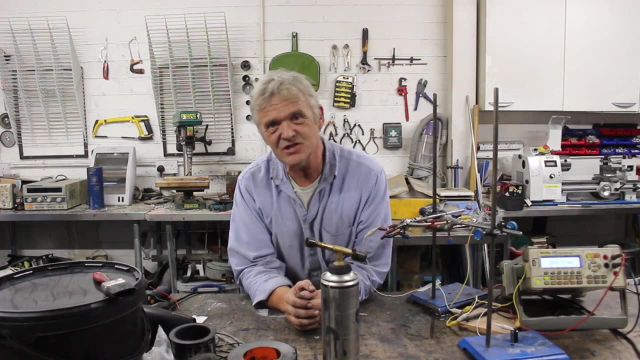 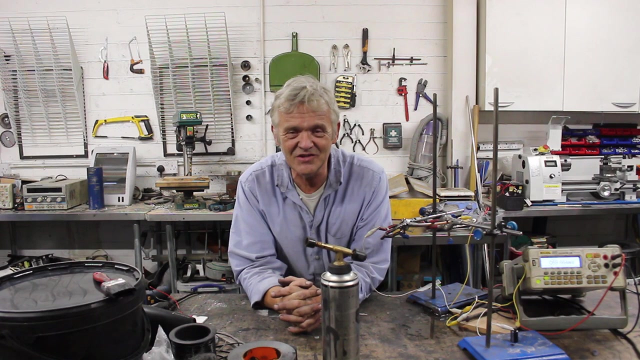 three. so we are actually pumping charge out of this arrangement into that capacitor. So we used magnesium because that's what we've got. but the magnesium antimony alloy apparently performs even better than that and there is a plan to put it on the Mars Rover to be a heat generator. for that It was certainly 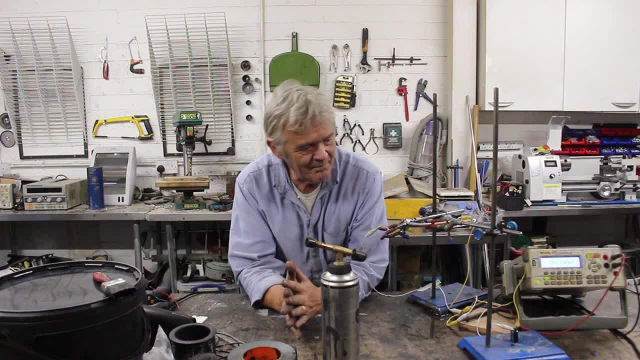 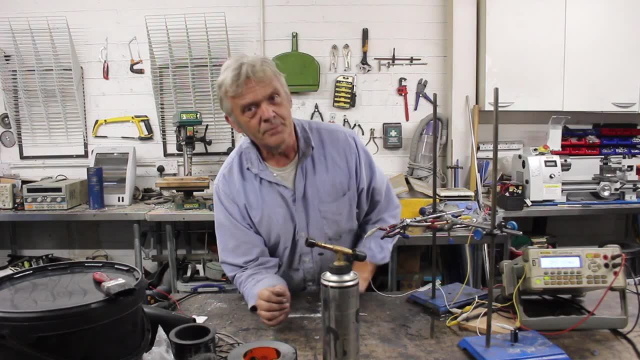 very impressive and I wanted to share it with you because a lot of the times, it's these weird combinations of materials that can give the results you're looking for. I used a bit of copper because, again, it's easy to use, but you might want to try nitinol, you might want to try constantan. 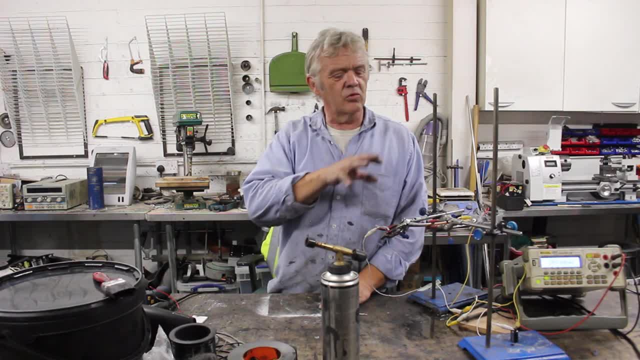 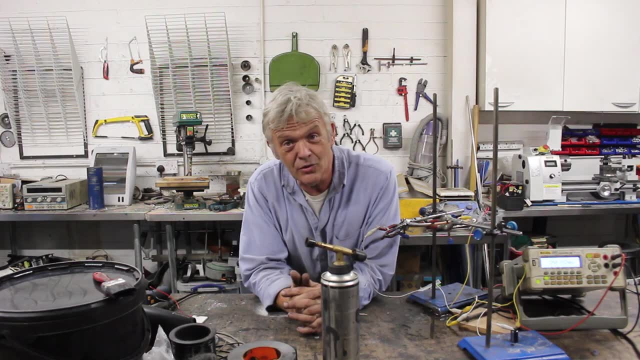 something like that, Or cancel even. There'd be a whole range of materials. you could try Some way of doping. that magnesium might be really cool If we could work out how to get the antimony in there. then we'd be able to reproduce that material. but you can actually buy it Now one way to do it of. 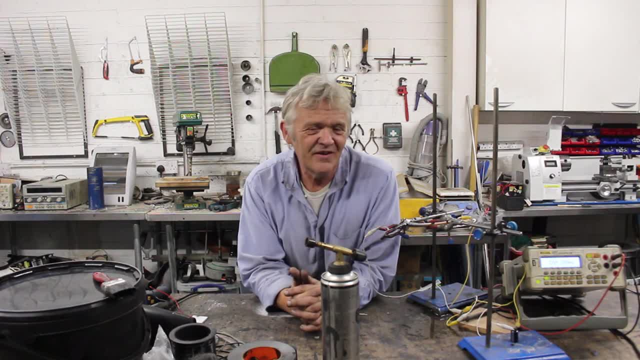 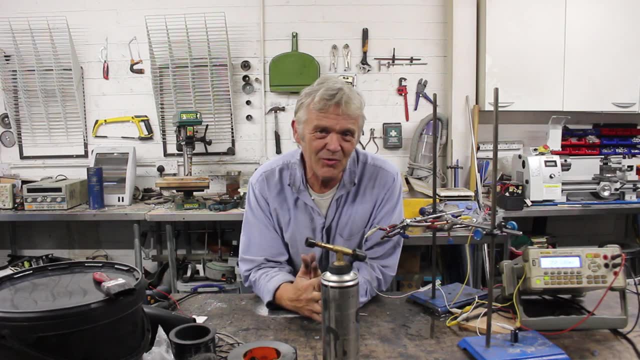 course is to ball mill magnesium powder with antimony powder and you'll form the magnesium antimony. Anyway, I thought I would share that with you and the news that the thermoelectric junctions have just made a huge leap forward. I hope you enjoyed the video. Thank you very much for watching and please do remember to like and subscribe.